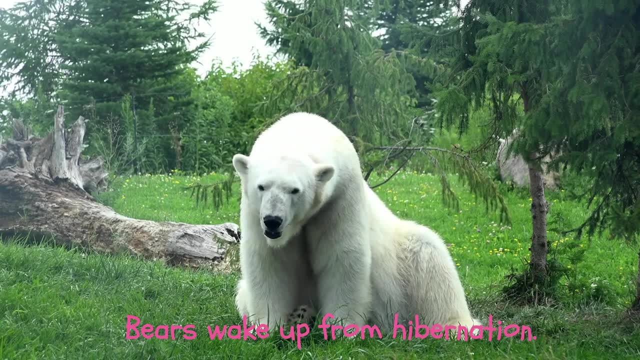 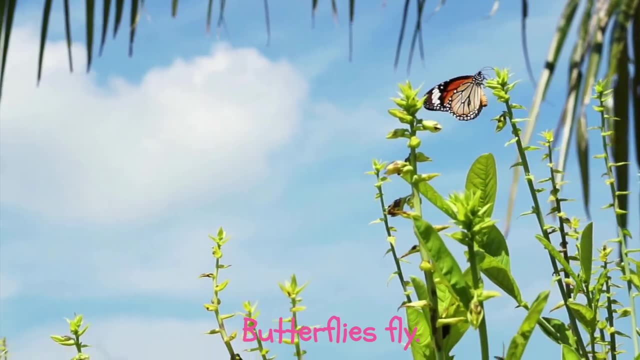 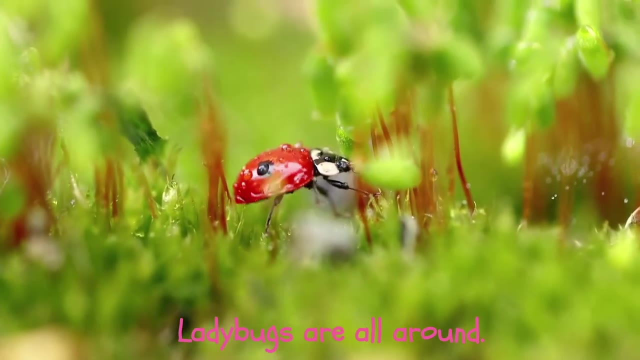 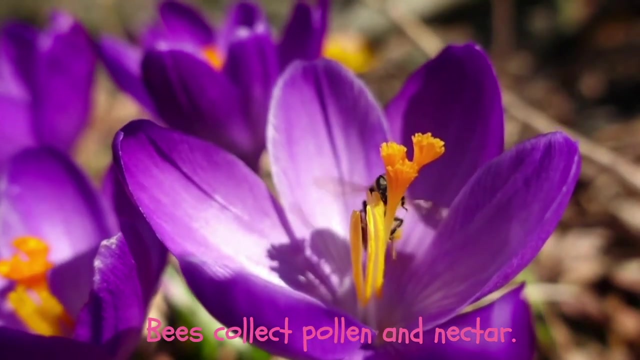 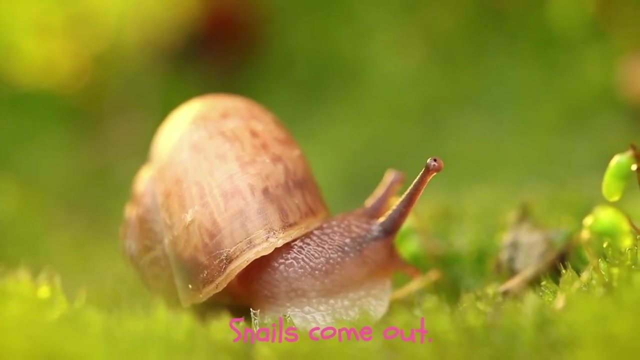 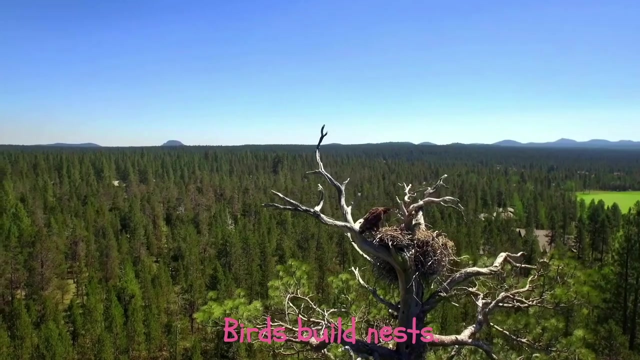 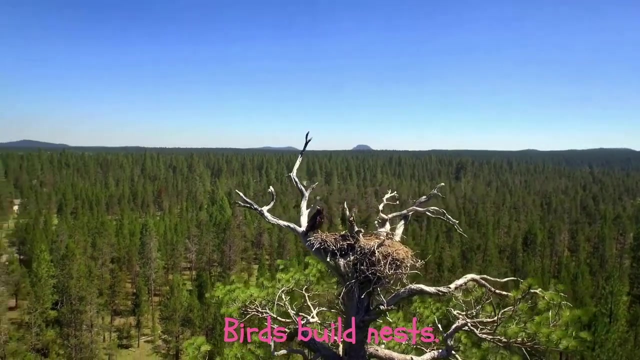 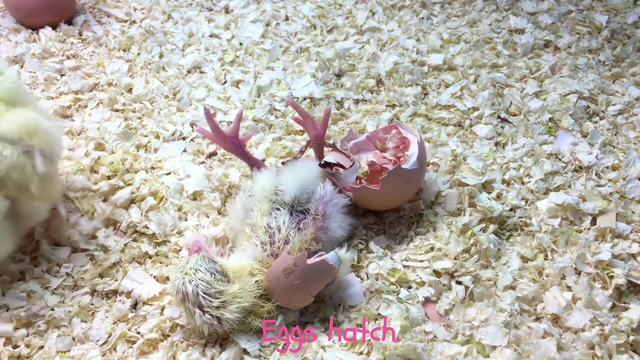 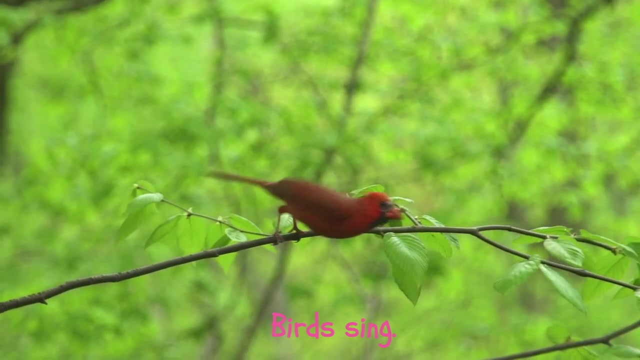 Butterflies fly. Ladybugs are all around, Bees can fly, Birds can fly. Bees collect pollen and nectar. Snails come out, Birds build nests. Eggs hatch. Birds sing Insects come out. Bunnies hop around. 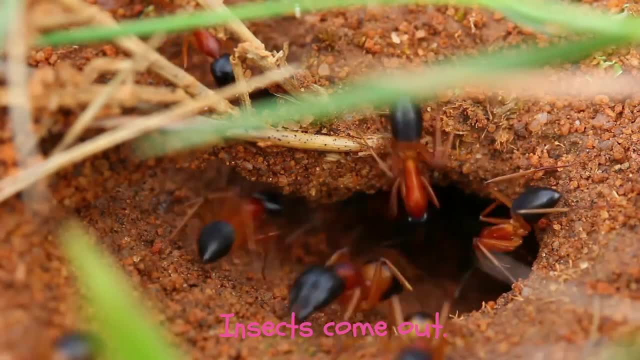 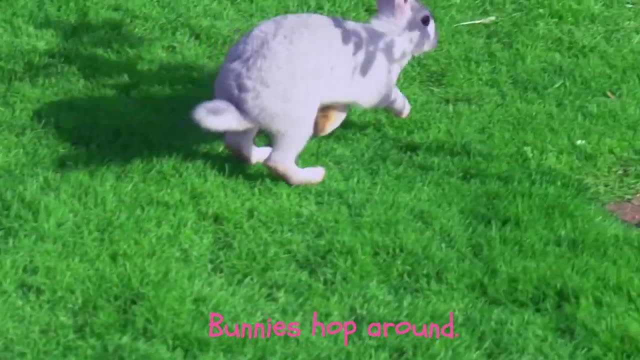 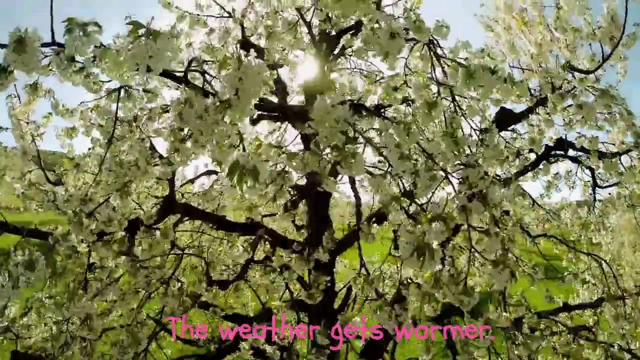 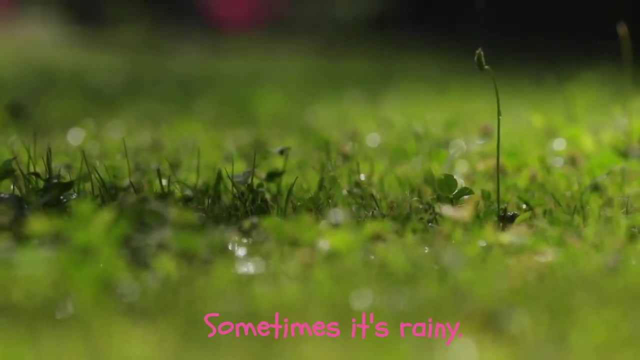 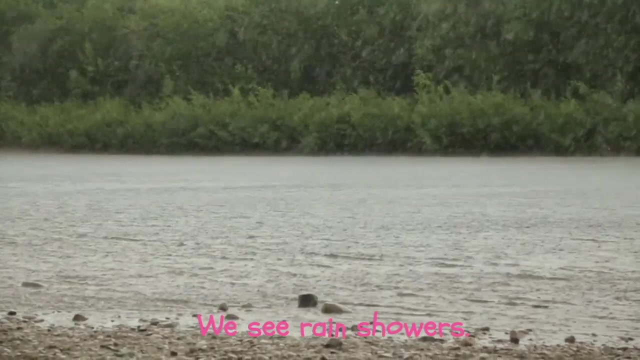 The weather is great. The weather is great. The weather is great. The weather gets warmer. The weather gets warmer. Sometimes it's rainy. We see rain showers. We see rain showers. We see colorful rainbows. We see colorful rainbows. 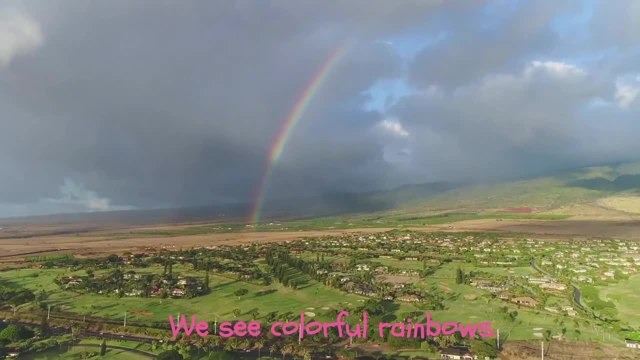 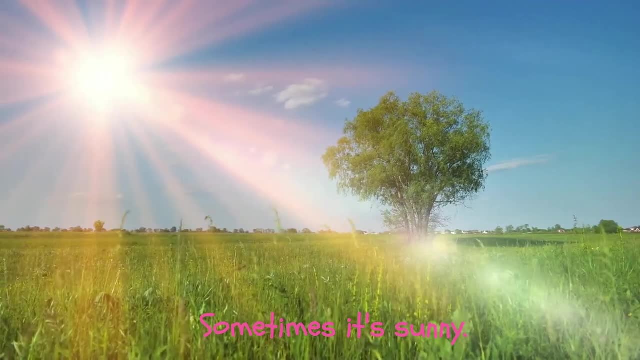 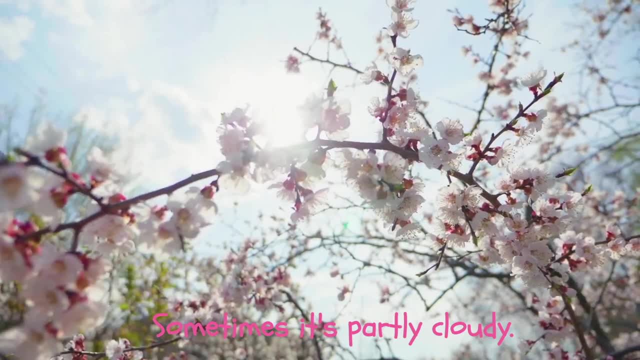 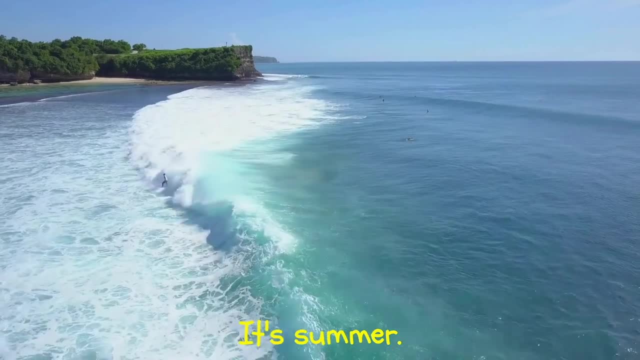 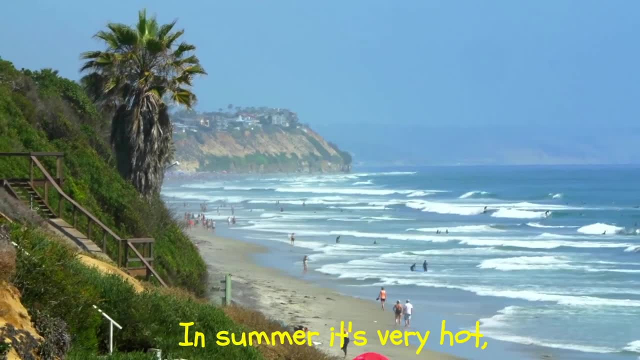 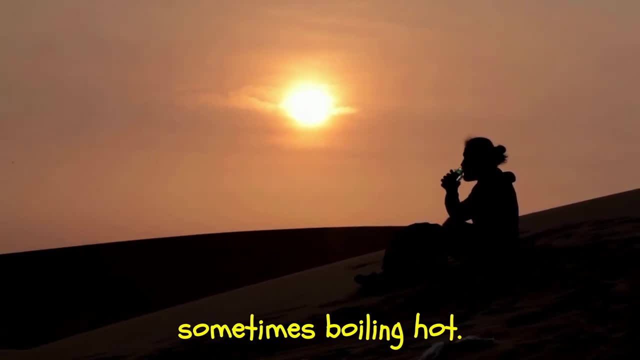 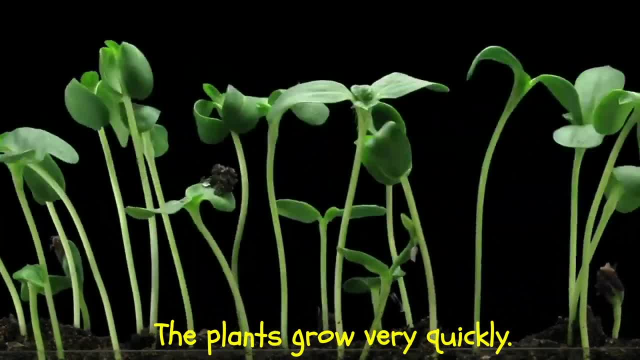 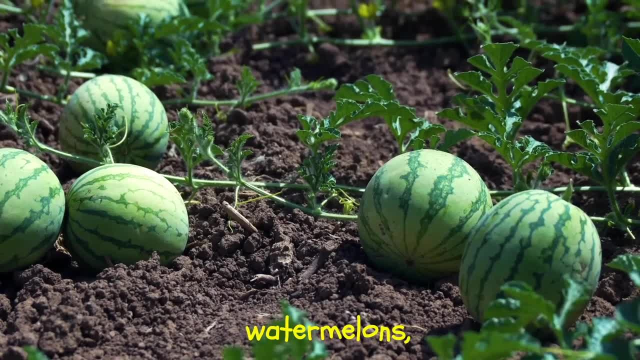 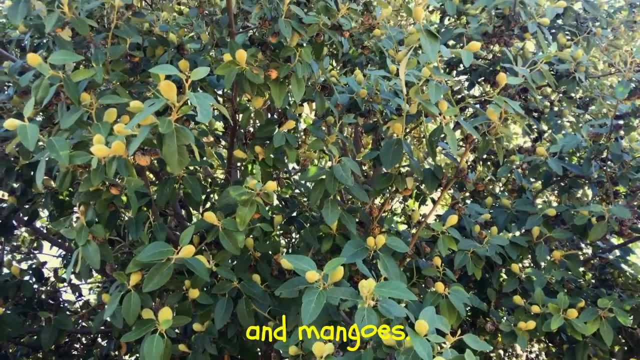 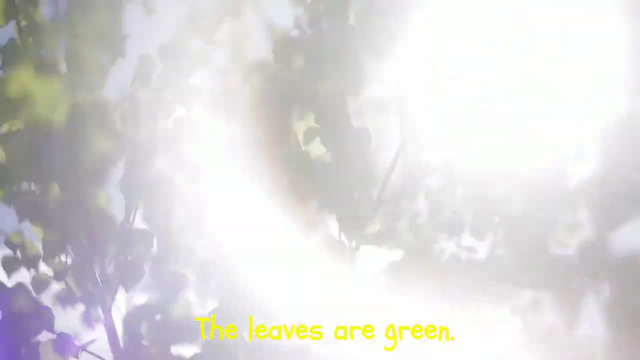 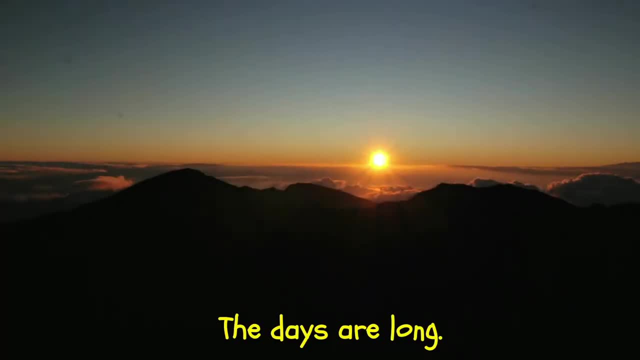 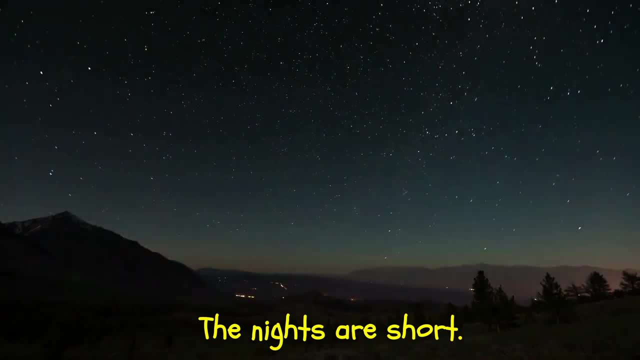 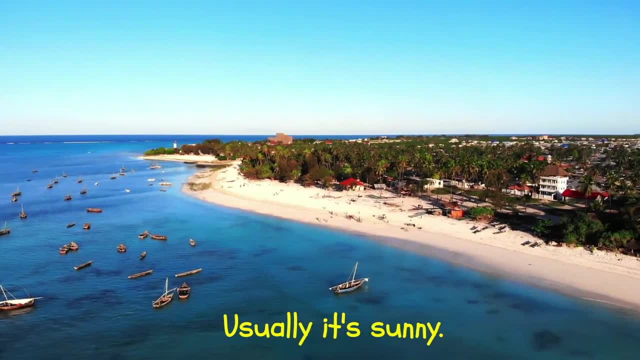 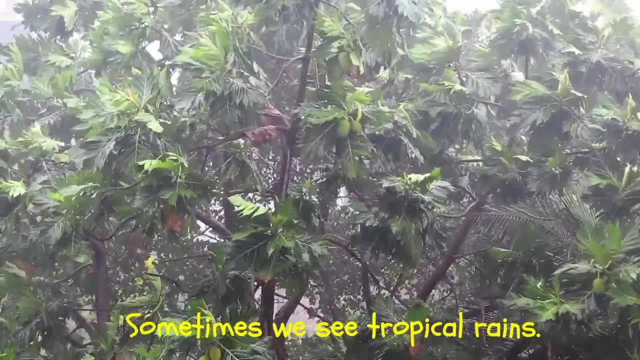 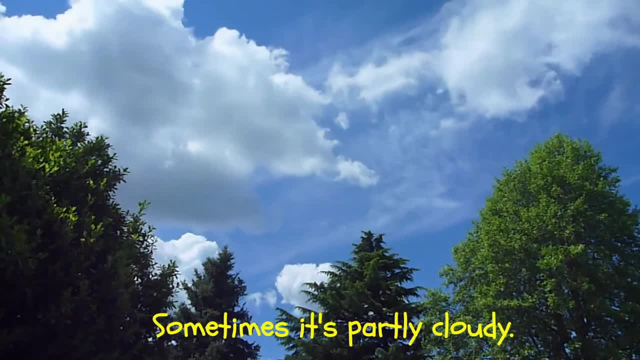 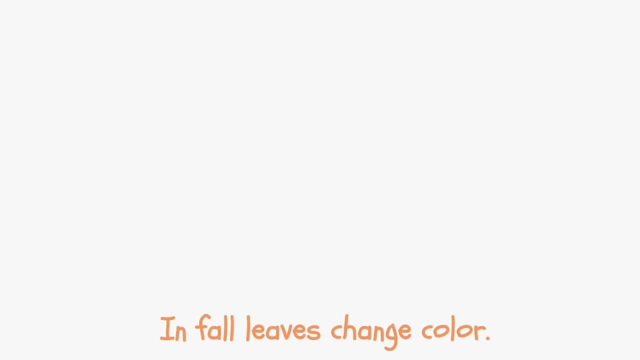 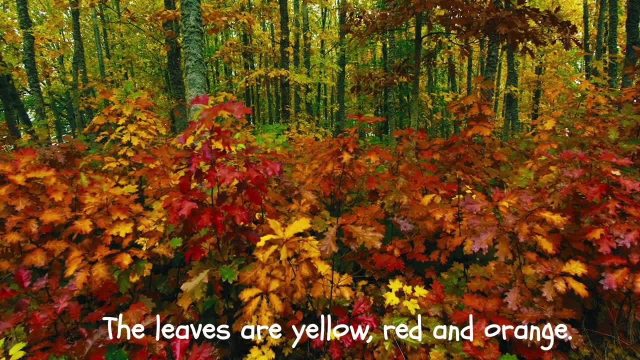 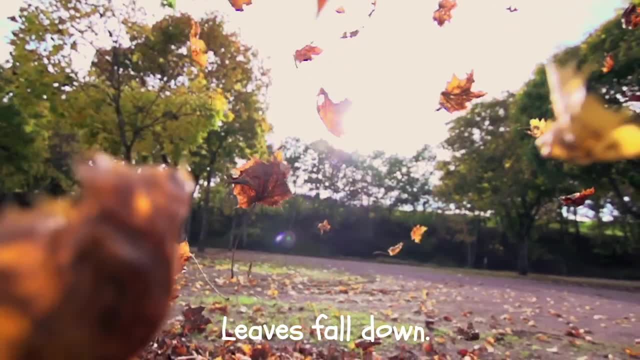 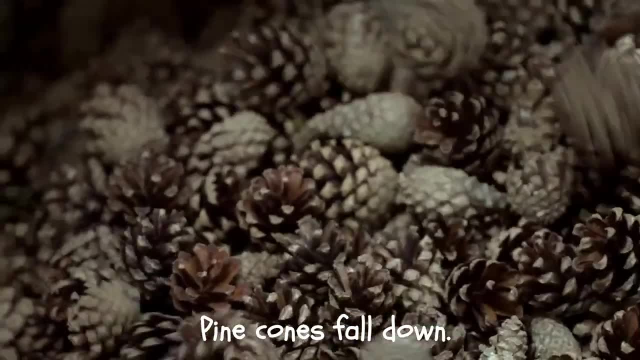 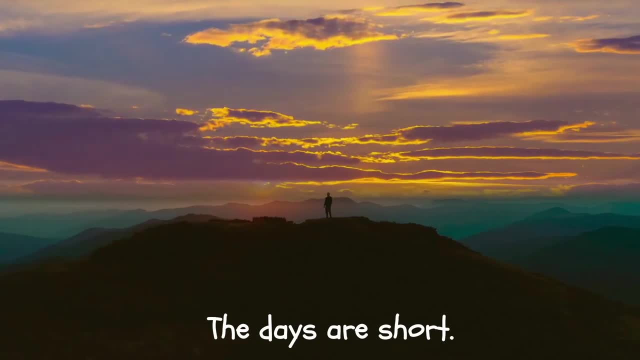 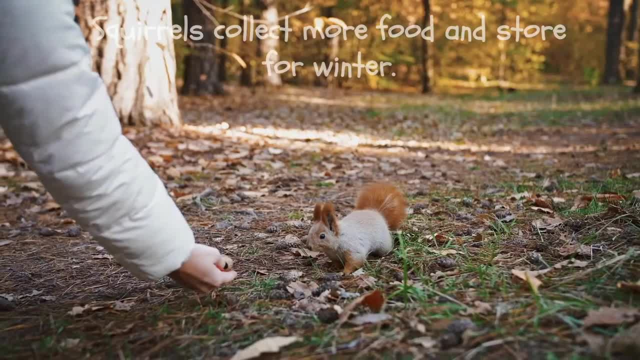 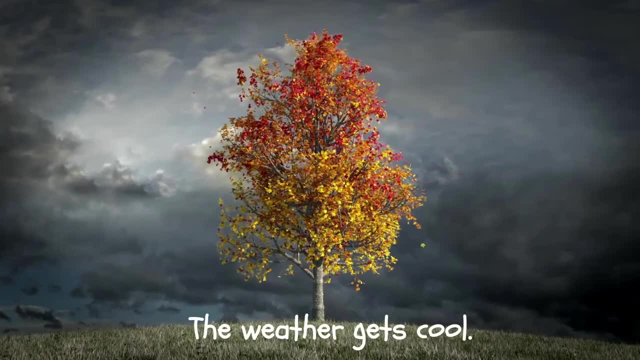 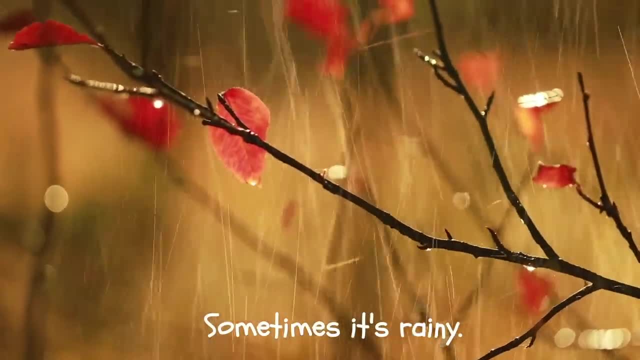 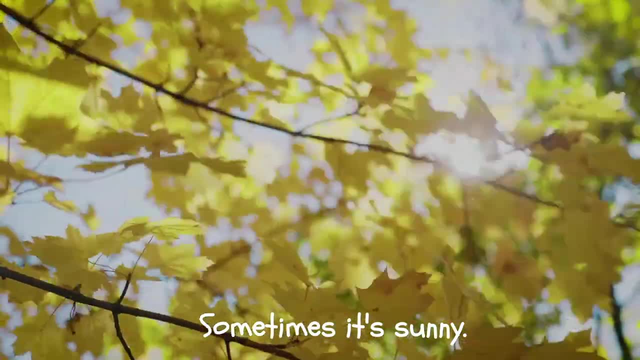 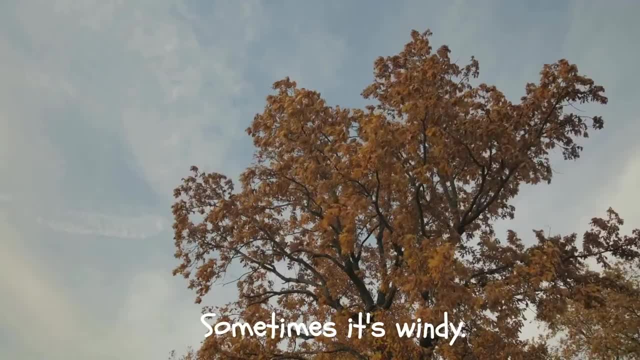 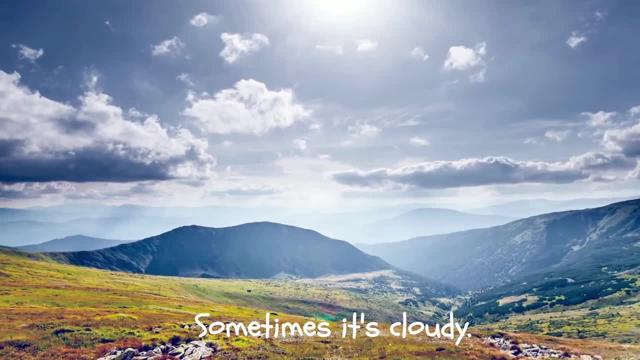 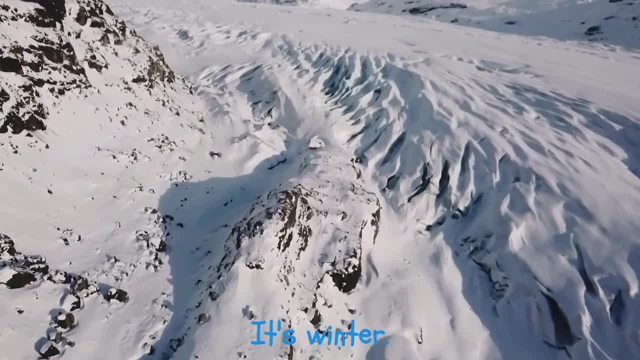 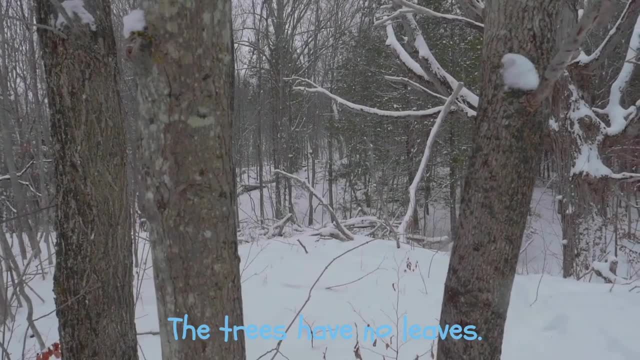 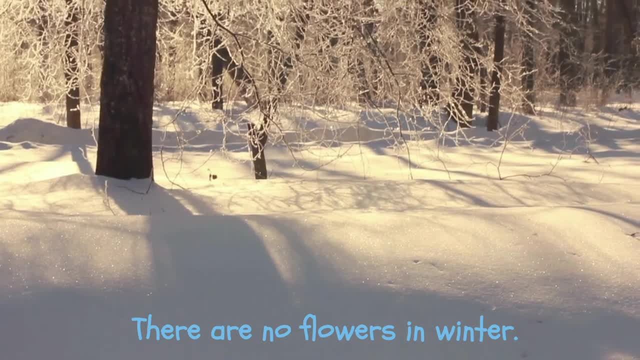 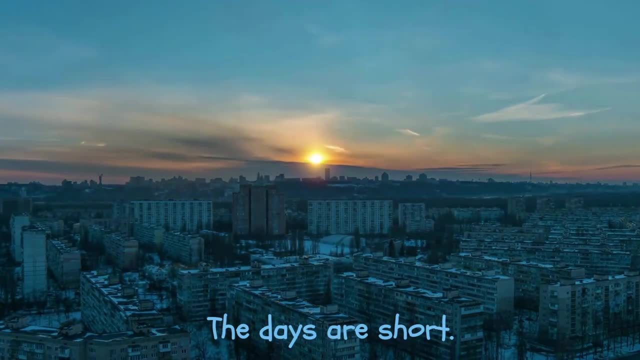 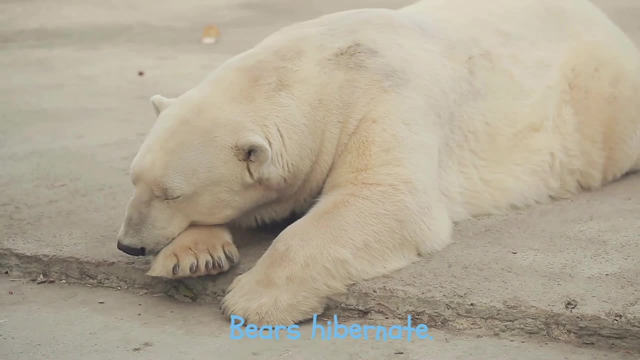 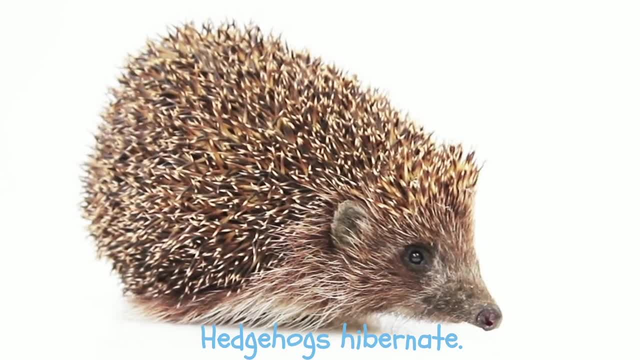 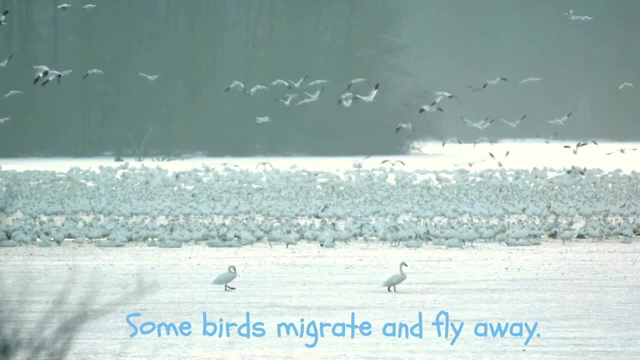 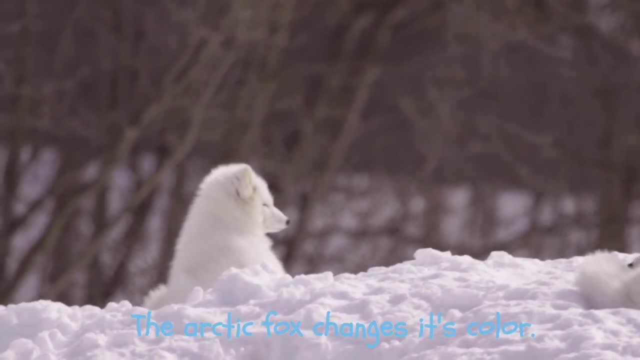 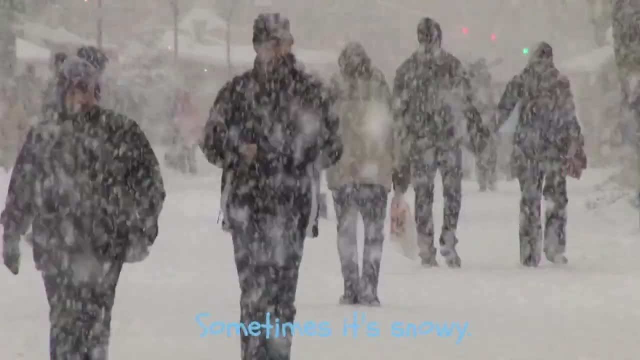 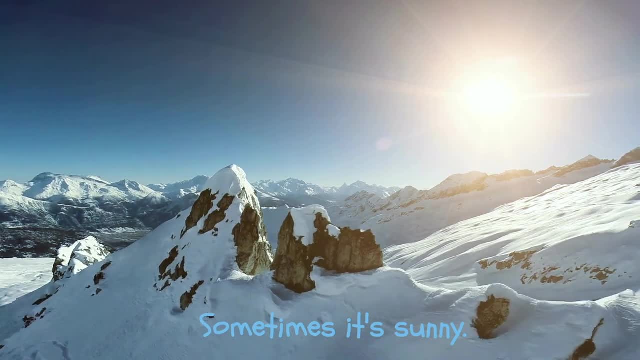 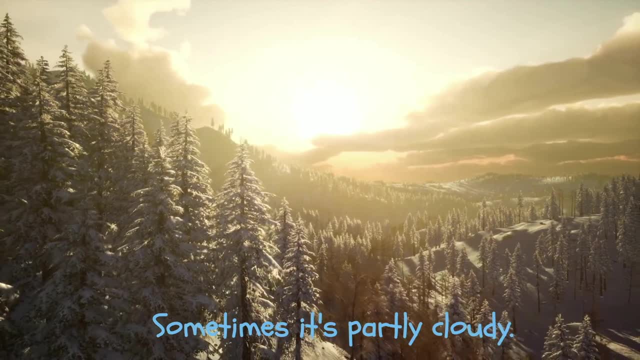 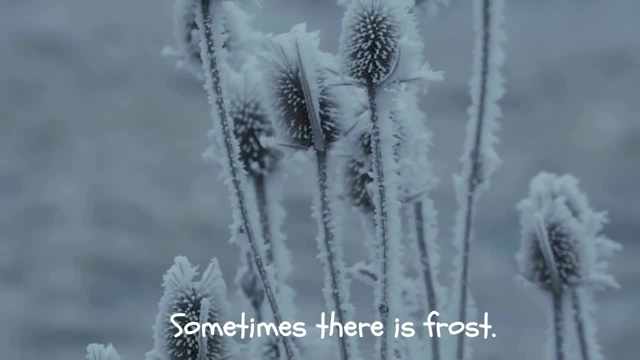